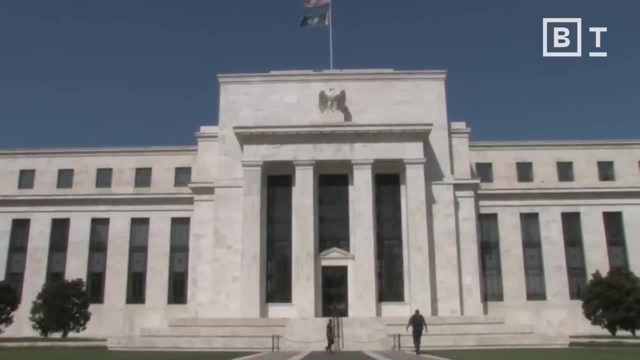 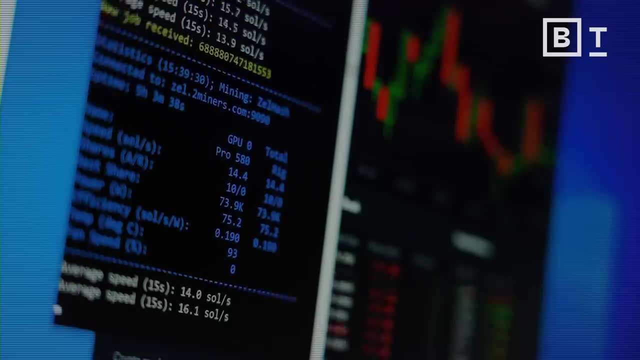 It cannot easily be overruled by an outside authority or central authority. So it's like you have at the same time potentially a new kind of money, A new kind of investment asset and also actually a new kind of computer. 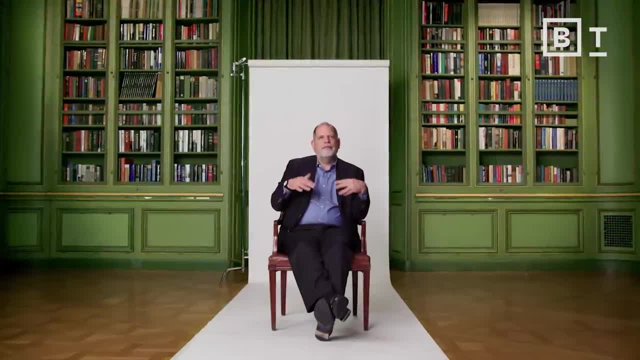 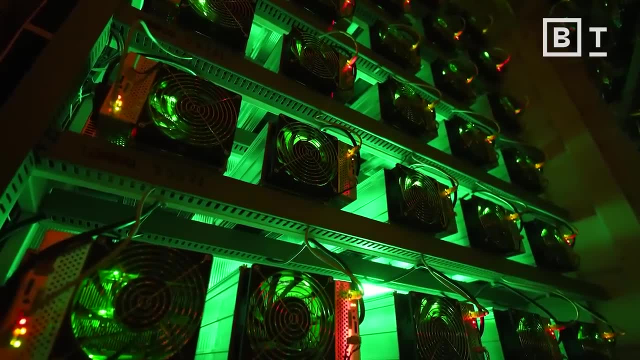 So when I talk to people who are deeply into crypto, I often feel quite skeptical. They have such bold grand plans and I'm not convinced they've thought through how to carry it all out. At the same time, I know many people who dismiss crypto altogether. 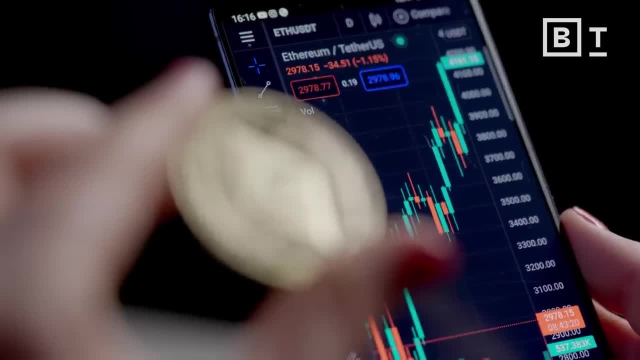 They think it's a scam or a bubble or a fraud and when I talk to them I feel quite bullish about crypto. I see a lot of potential in the ideas, but I don't think we know yet how useful crypto will be. 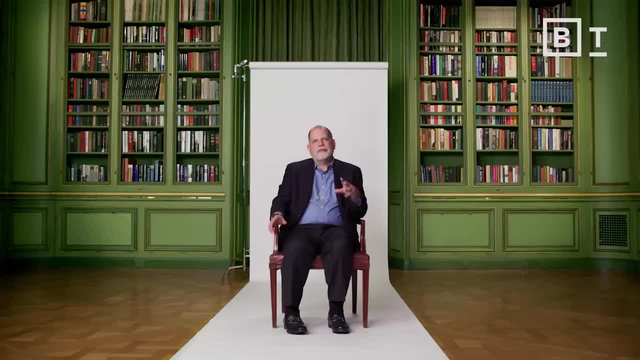 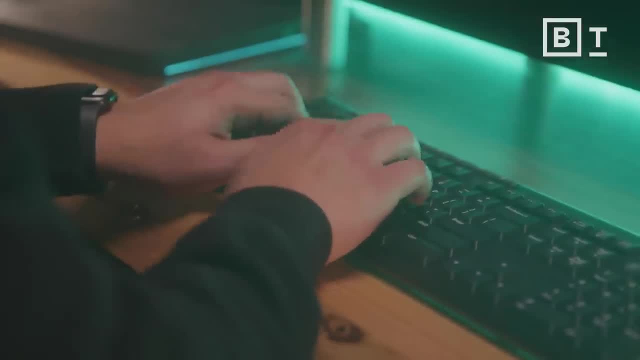 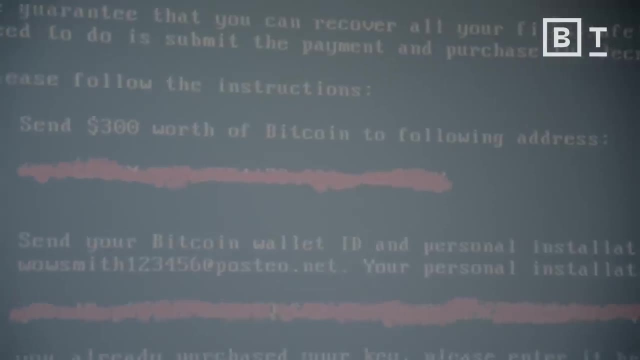 Here are some reasons why the crypto skeptics are skeptical. People use crypto to pay off ransoms. that say, hackers will go into the medical records of a hospital, pull out or lock or freeze that information and they won't give it back until they're paid off in crypto. 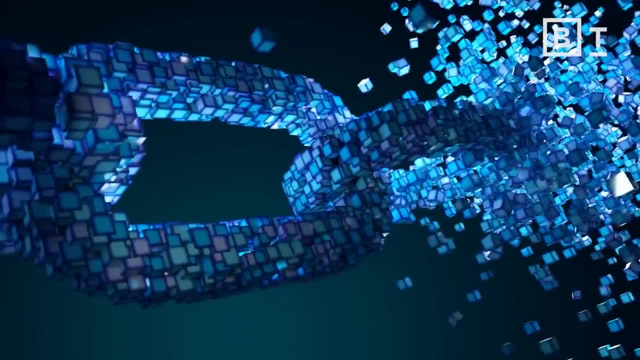 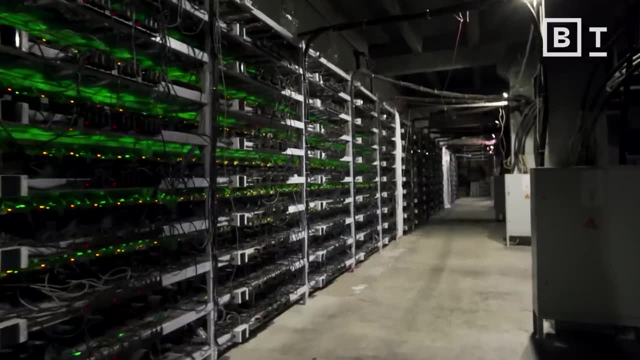 You can't ever get your money back. It's an irreversible transaction done on the blockchain. That's the end of it. Crypto itself, in most of its current forms it, consumes a lot of energy. You have computers racing to make calculations, to crack different kinds of cryptographic. 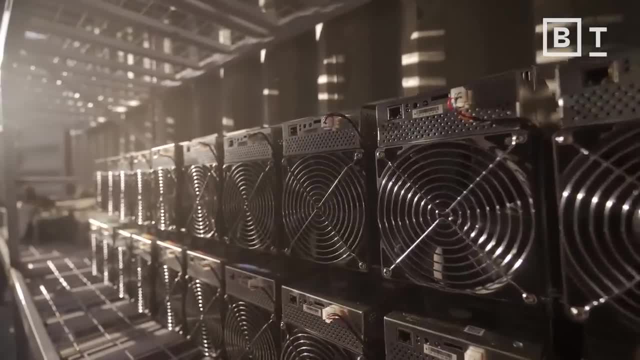 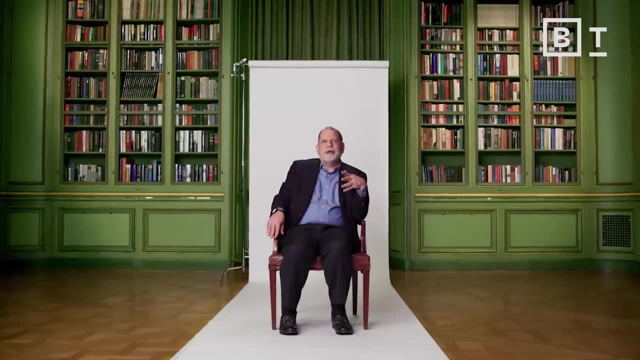 problems, and those computers use so much energy that it damages the environment through carbon emissions in a way that we understand pretty well now. But maybe the biggest reason to be crypto skeptical is simply that a lot of the promised benefits haven't happened yet. Well, it's going to make banking cheaper. 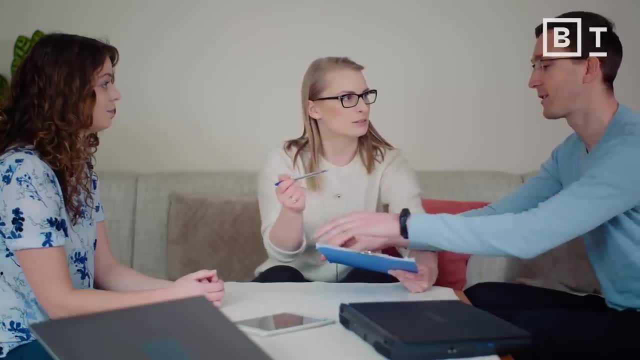 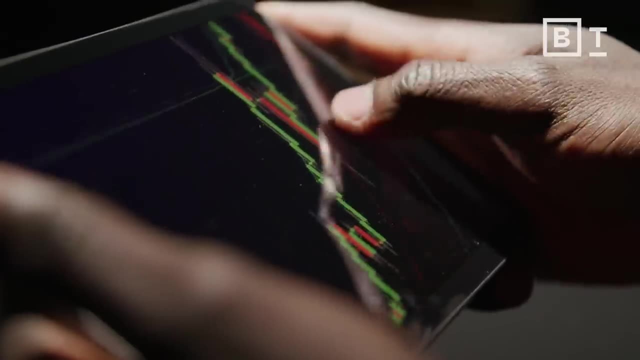 It's going to make finance cheaper. It's going to make lending cheaper. Maybe those dreams are just impossible, or impossible anytime soon. I don't know. I don't know. And if people are skeptical about the promised benefits of crypto, they have some good reasons. 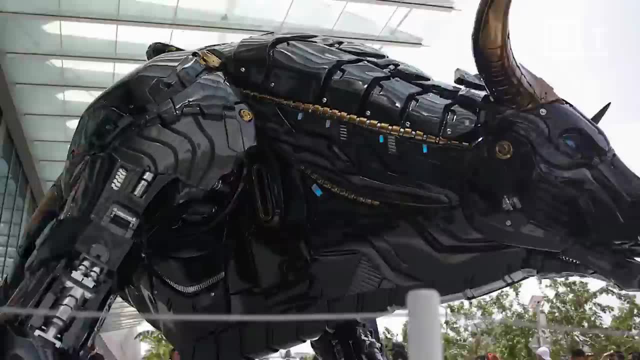 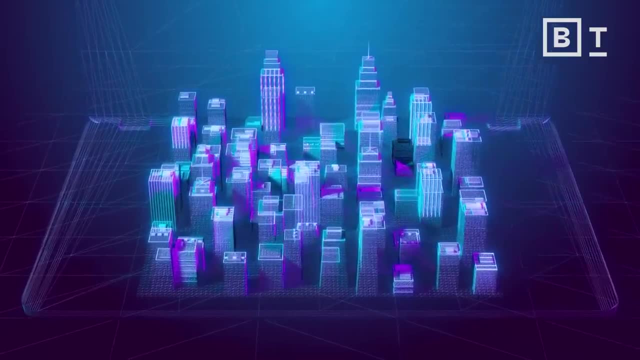 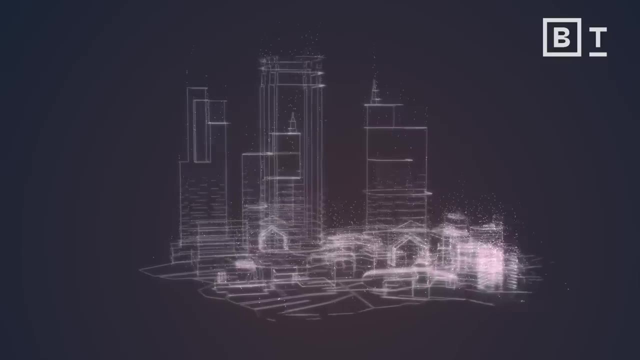 to be skeptical. Here's a way to think about the bullish case for crypto. Imagine that the internet becomes more and more its own economy, with its own series of rules, and that economy is a global one. It will need its own systems of record keeping, its own systems of property rights, its own.